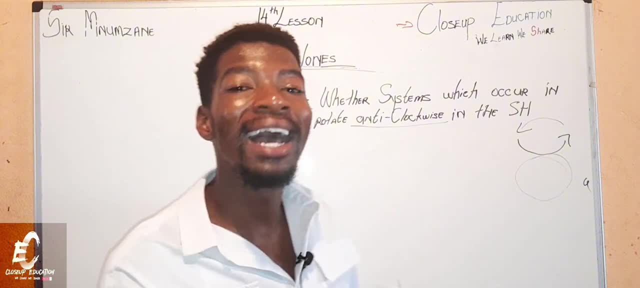 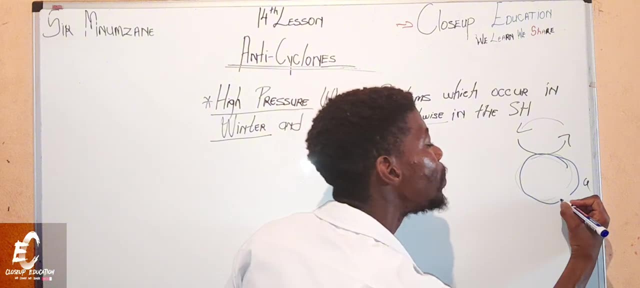 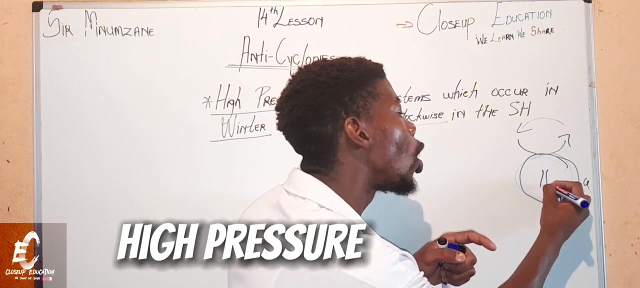 this is our isopar. what is happening to our marker? let me use another one. this is our isopar, right? so when our isopar reaches a thousand upwards, you must know that inside here there is what we call high pressure. this is high pressure from thousand hectoparts. 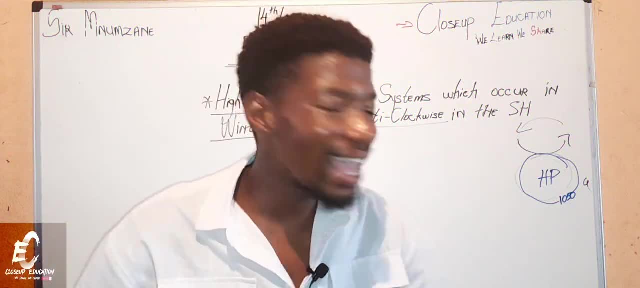 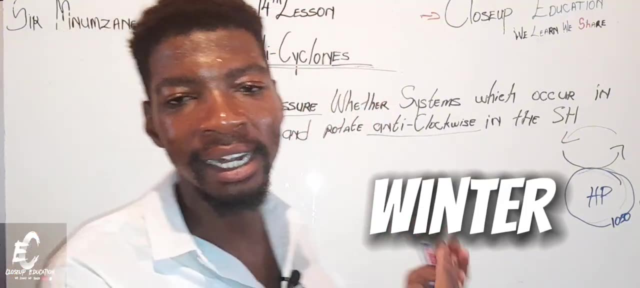 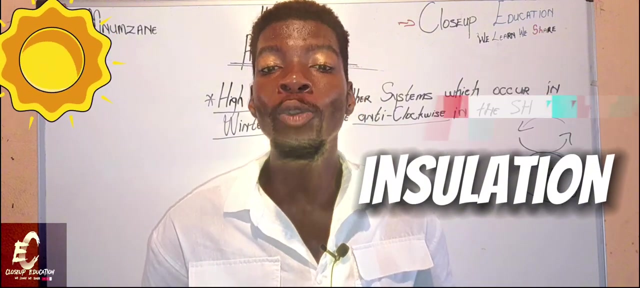 pascals calculated. now we know that there is high pressure. all right, let's continue. we must remember that we are talking about the winter season, meaning our ocean and our land is not receiving any direct insulation, or we could say enough insulation from the sun, meaning we will not have. rising or evaporation, because of the air which is on our ocean and our land is not directly insulated or heated up by our sun enough, because of we know that it is winter and in winter we have obviously what we call shorter days and longer nights. that's why you might find 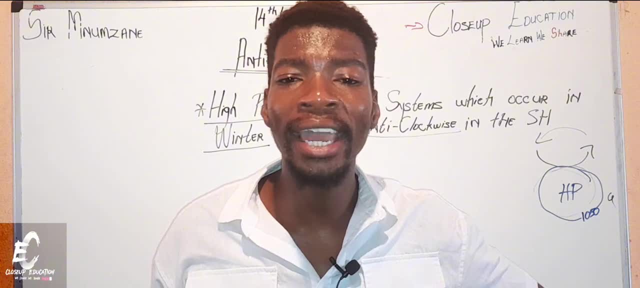 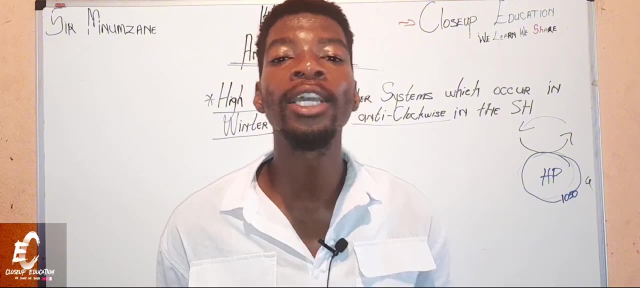 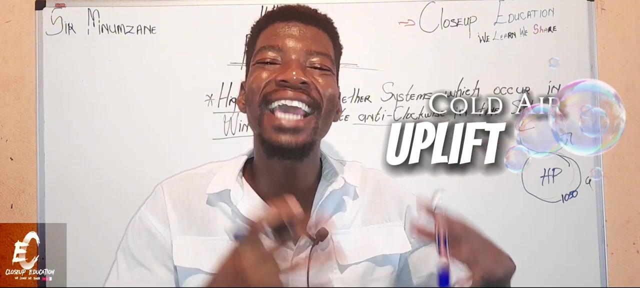 yourself sleeping. oh, what the heck. it is already seven and i'm still sleeping. yes, that is winter, meaning our land and our ocean are not receiving enough insulation from the sun, so there won't be too much evaporation to be able to have解放 able to uplift any air, so they will be obviously sinking air. so our area, which is obviously south, 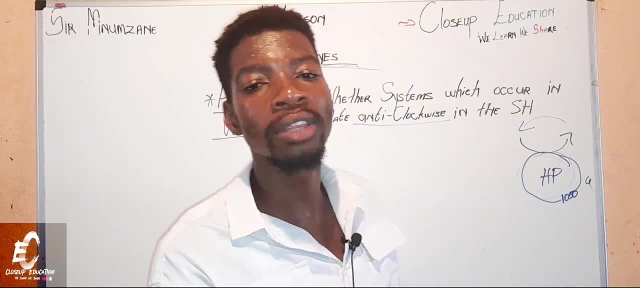 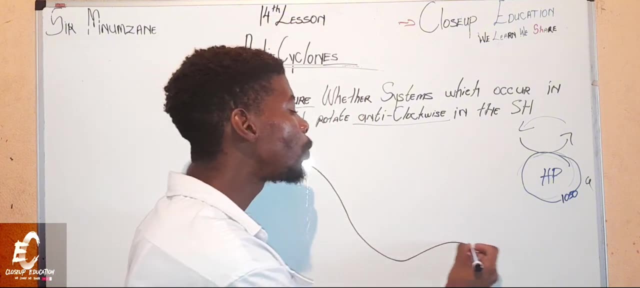 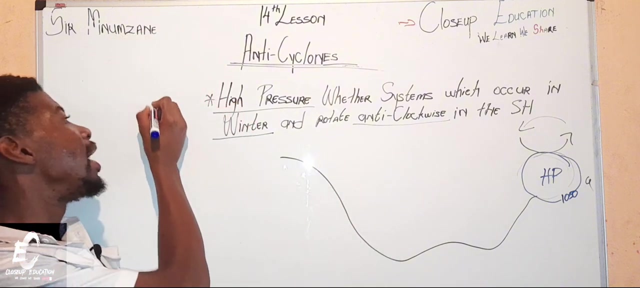 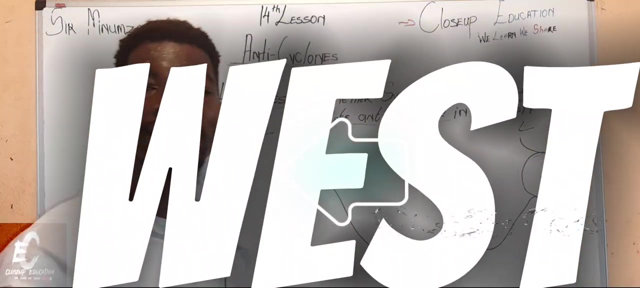 africa. i'm from south africa. we'll be using the map of south africa to understand what i'm actually teaching. okay, so this is obviously our what we call south africa, right in south africa. we know that this side, it is our obviously what we call a never eat sour west. this is side, it is our west. 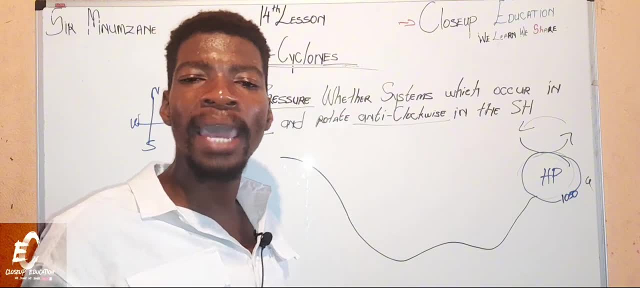 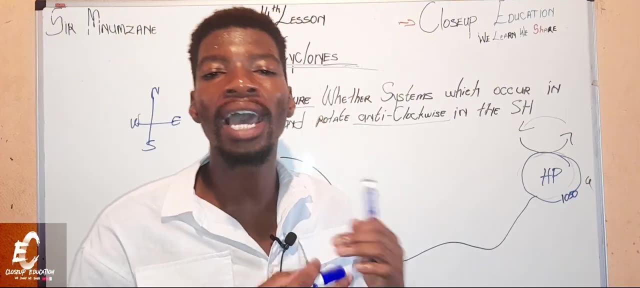 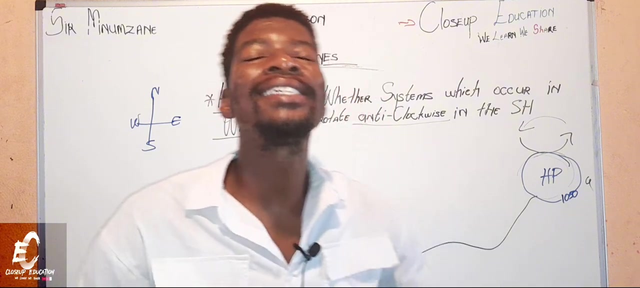 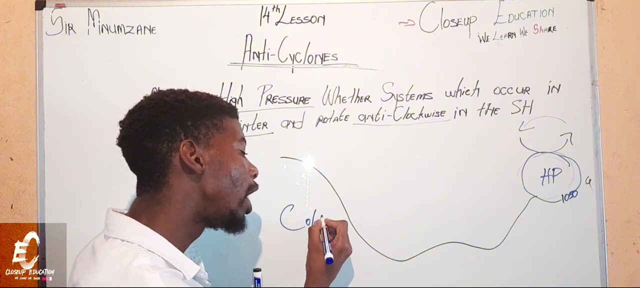 meaning. this is our western cape right. and in a western cape, which ocean do we find? we find the atlantic ocean. and what do we know about the atlantic ocean? we know one most important characteristic: that the atlantic ocean has cold ocean. it is cold, and in the atlantic ocean we know that it is what we call cold right. and what do we have? 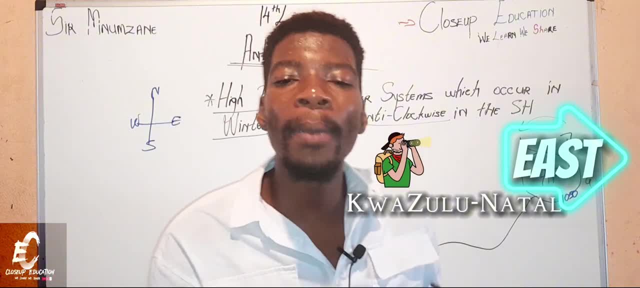 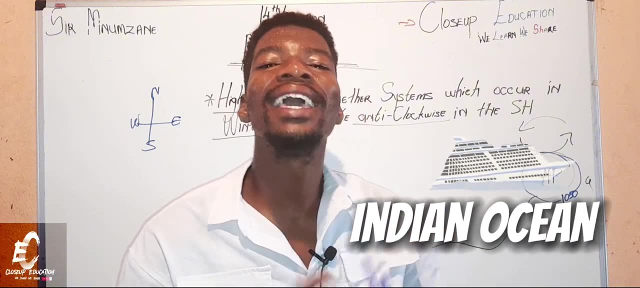 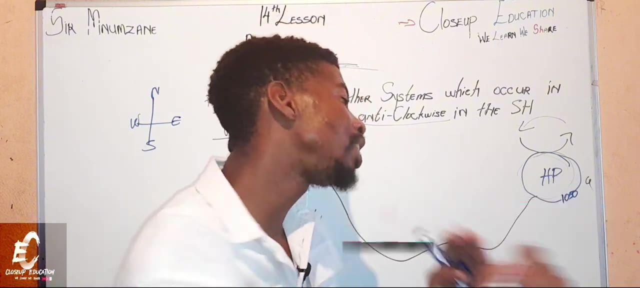 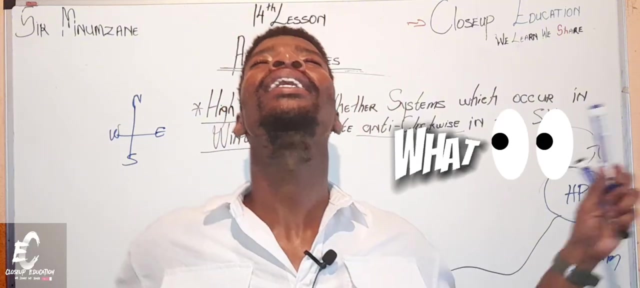 this side, our eastern side, we have debit. which ocean do we find in debit? the indian ocean. yes, the indian ocean. what do we know about the indian ocean? we know that it is warm. it is the warm ocean, right, so this is our warm ocean. okay, so now to better understand what the synonyms are saying, we have to know that there are three. 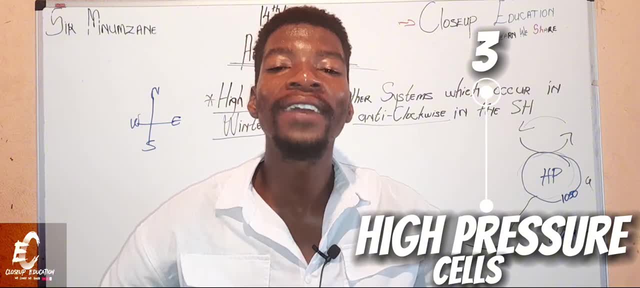 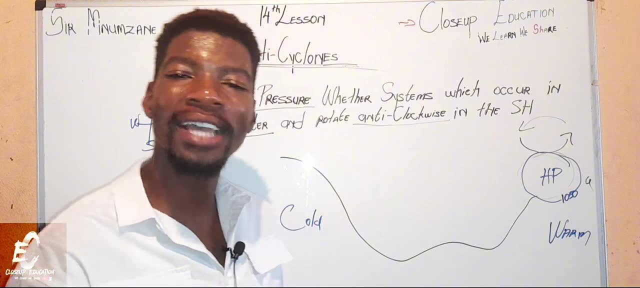 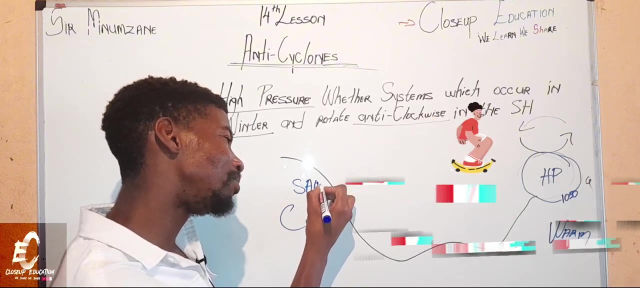 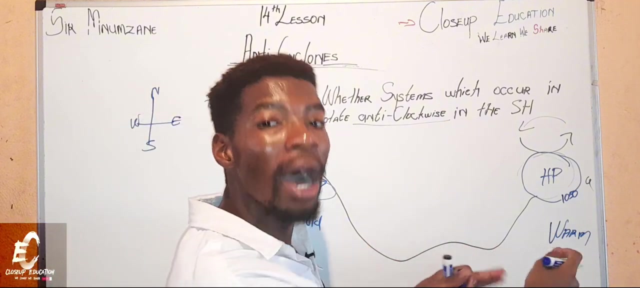 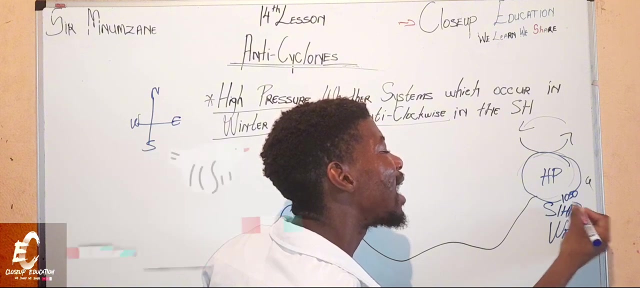 high pressure cells which affect south africa during winter. not one, guys, three high pressure cells which affect south africa. so what do we have here? we first have here our south atlantic high pressure. so this is our first pressure right, which is on our western cape side. then on our eastern cape side we have what we call our south indian high pressure. 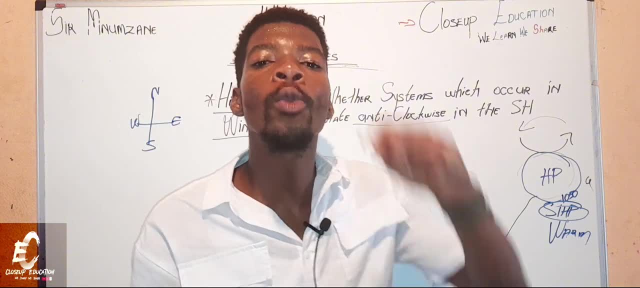 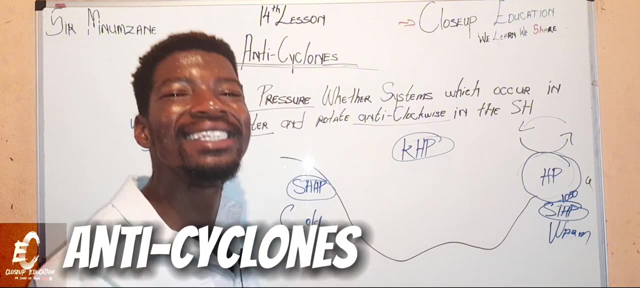 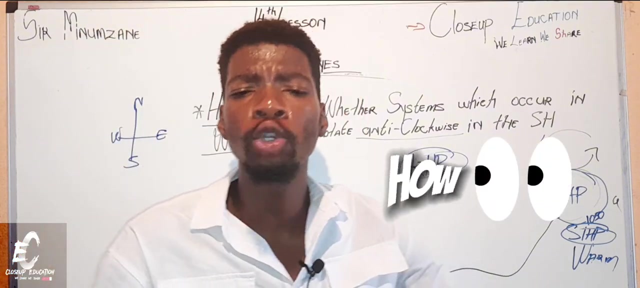 right, this is what we have. and not to end there, we also have what we call our kalahari high pressure. these are the three anti-cyclones which affect south africa in winter. all right, so how do they actually affect south africa in winter? we must know that they are very Klarahari, which means high pressure. 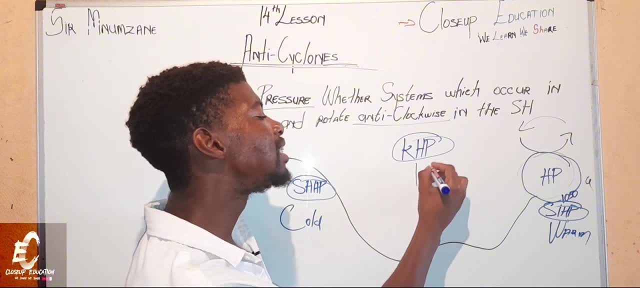 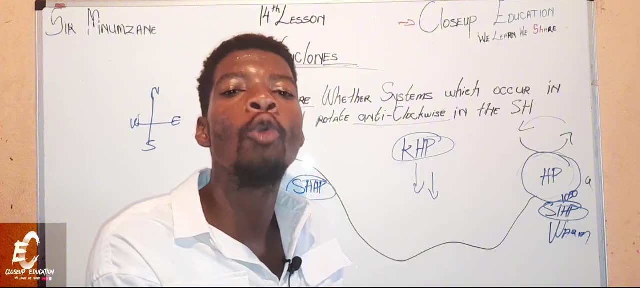 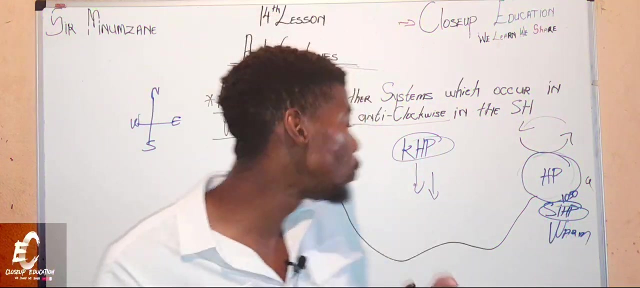 know that in winter we obviously have what we call descending, what we call descending air. this air, it is descending and it is cold, right, so we have descending air on our land. let's not move to our kalahari first, let's move to our south atlantic high pressure band. so if our air, it is descending, 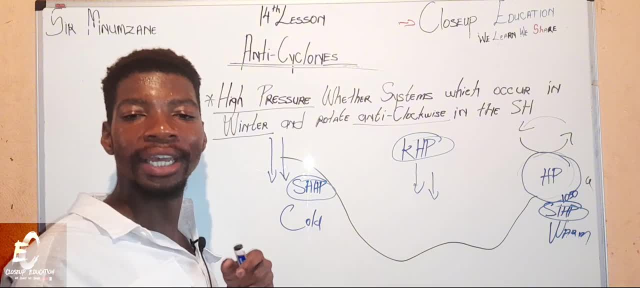 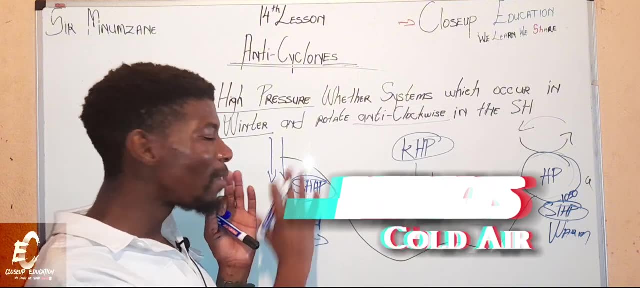 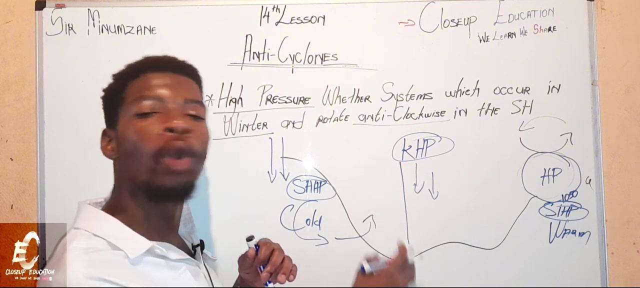 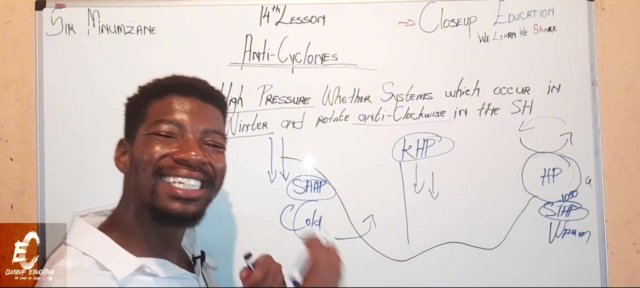 on our obvious cold ocean. it is obviously going to obviously do what deflect the cold air coming from the ocean into our land. right, and this area on the western cape will obviously experience cold conditions, so cold air will be deflected anti-clockwise into our land. so what is this? 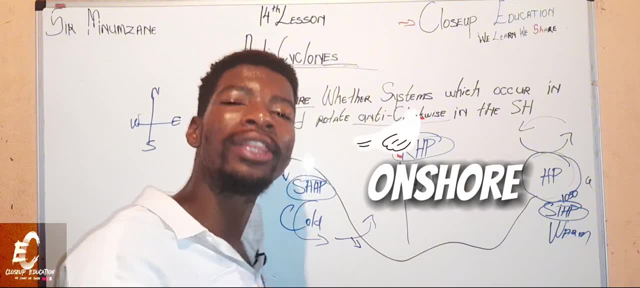 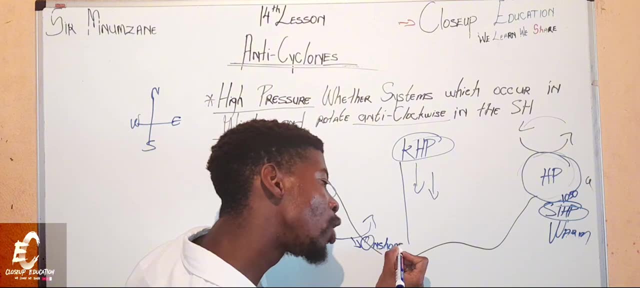 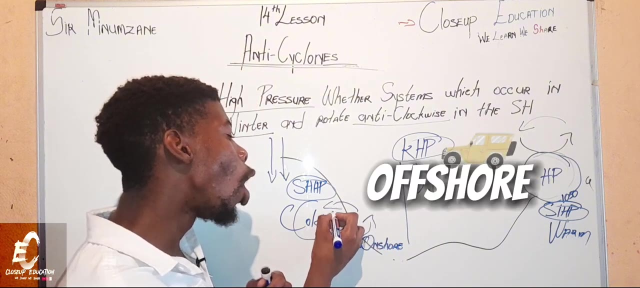 cold air that was deflating on our land deflector. it is usually called the onshores, right, so the onshores, because of it is entering our land. so these are the onshores and these are what we call offshores. all right, guys, we have to pass. 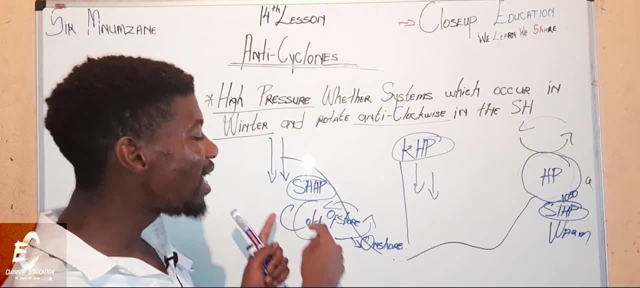 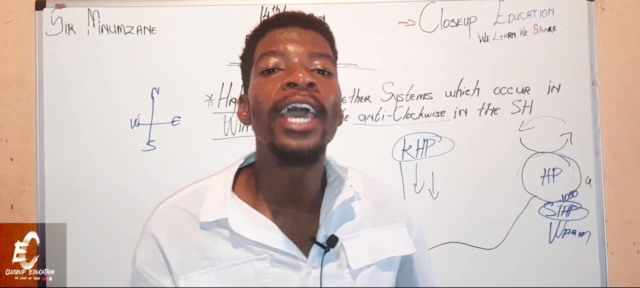 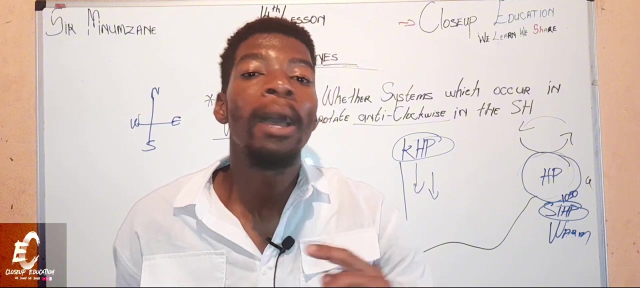 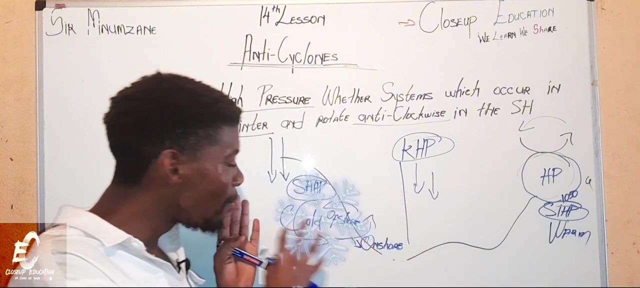 our metric. okay, let's continue. so this area, the western cape area, will experience cold condition, meaning, my guy, you will have to try and put on a bit of more what we call jackets, not one, but maybe even three when it comes to a western cape. western cape feels the cold coming from the ocean into the land. 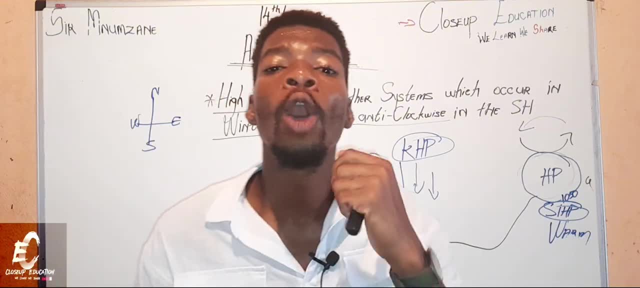 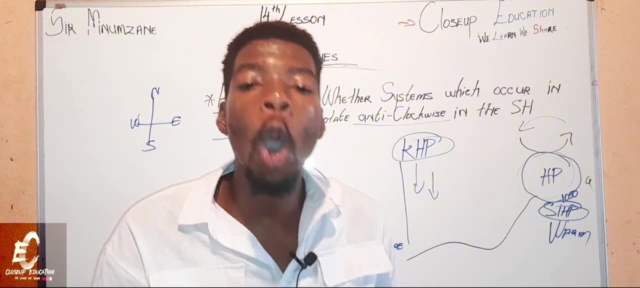 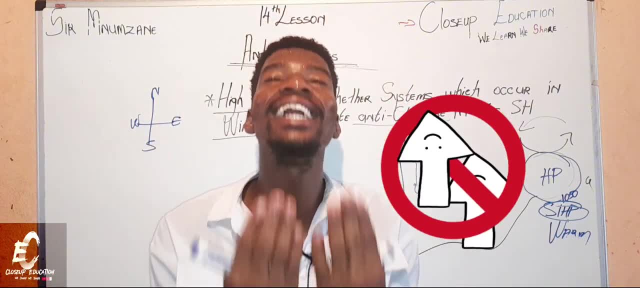 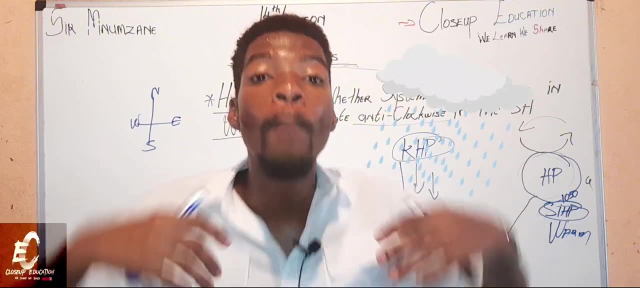 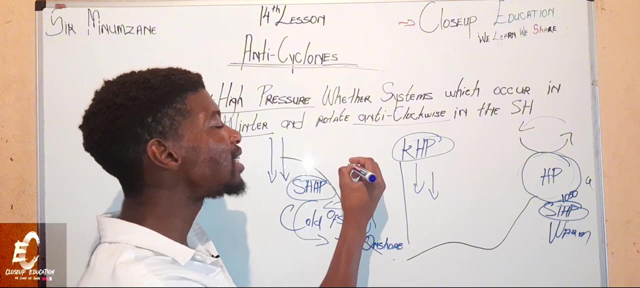 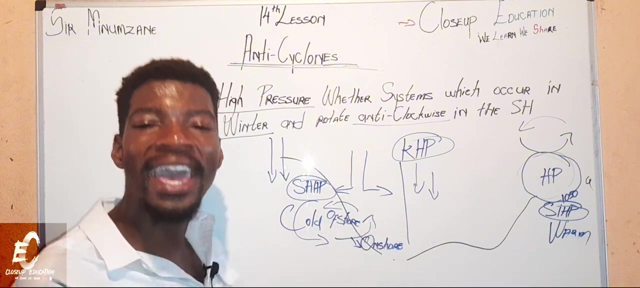 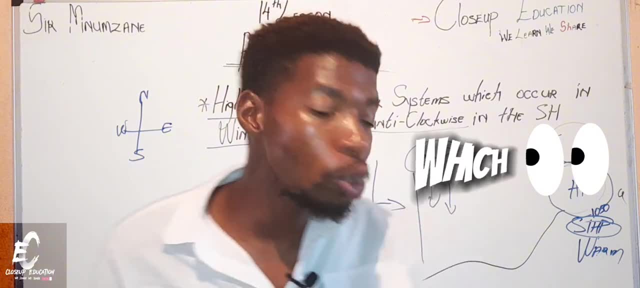 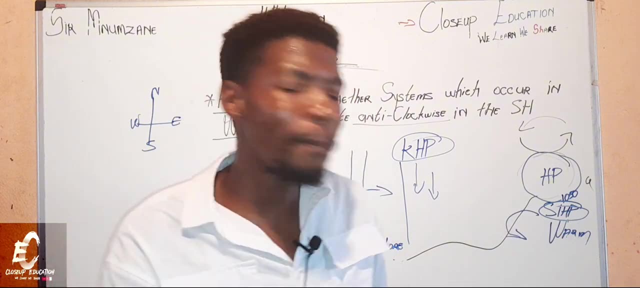 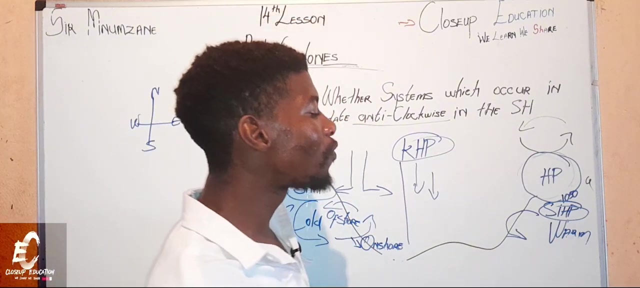 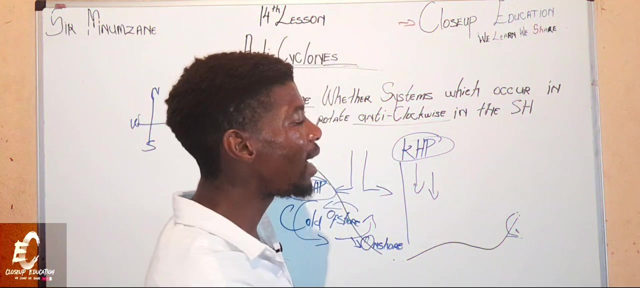 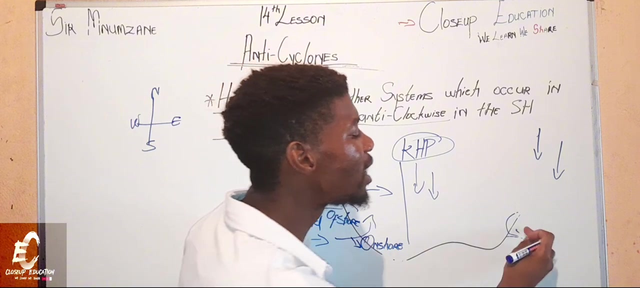 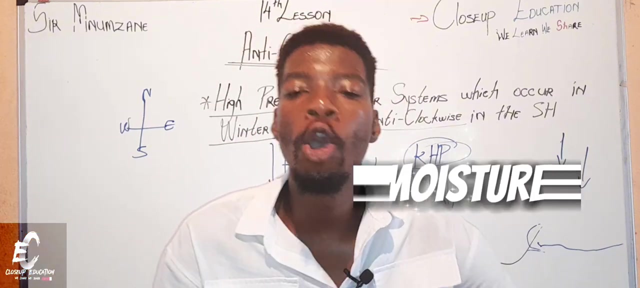 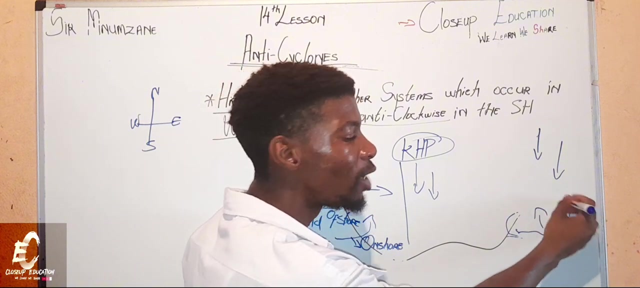 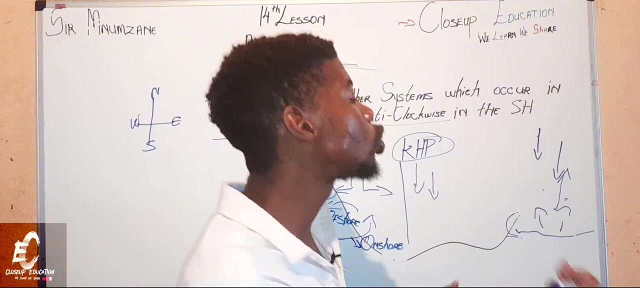 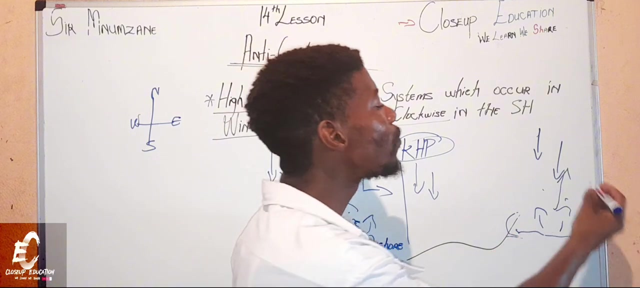 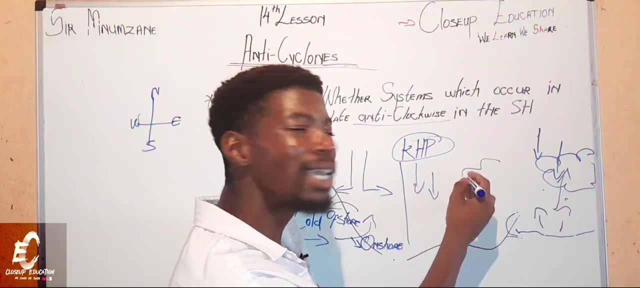 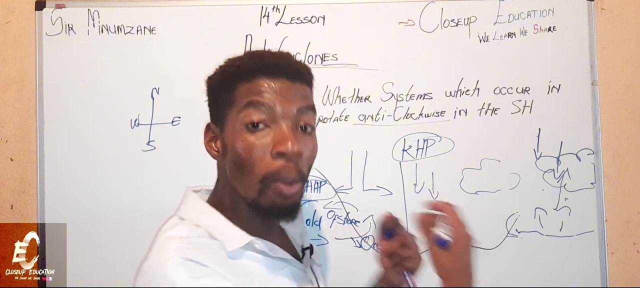 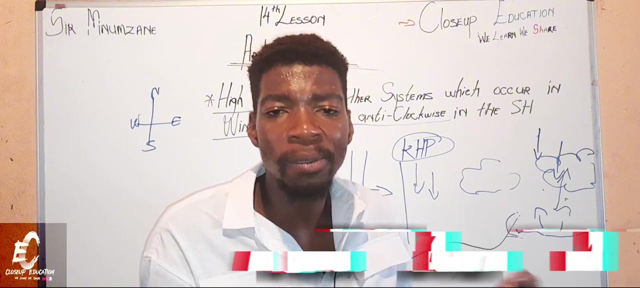 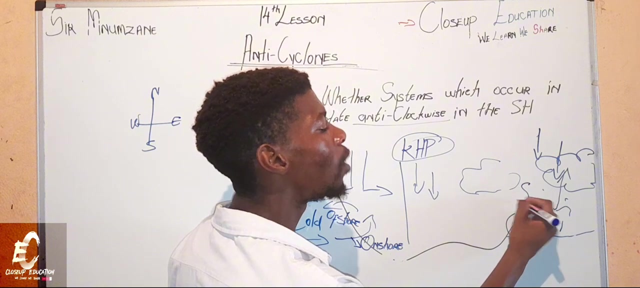 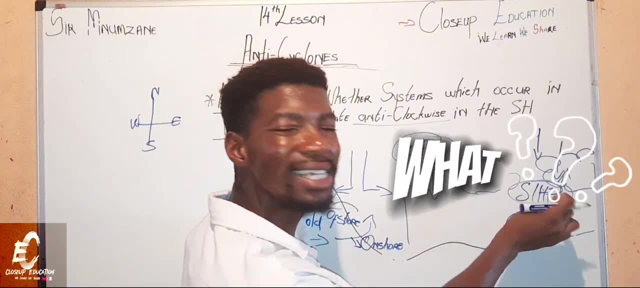 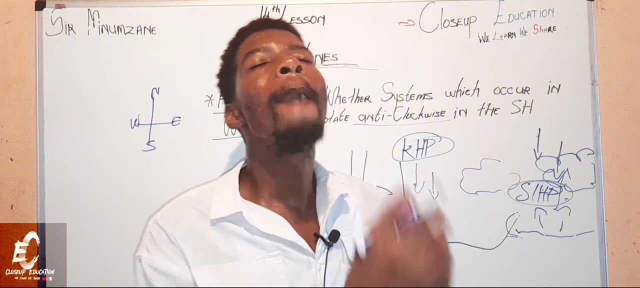 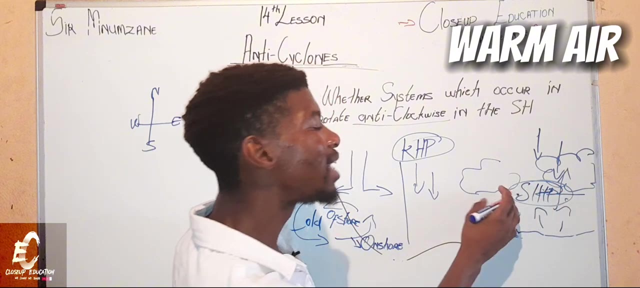 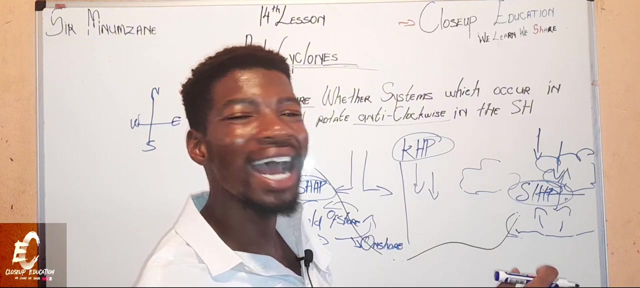 right in our south indian high pressure. what is this cell called this cell? it is usually given a name. it is also given a name. it is called our blocking cell, meaning it blocks a lot of moisture air from coming into our land to create a more evaporation and huge community member slugs. so 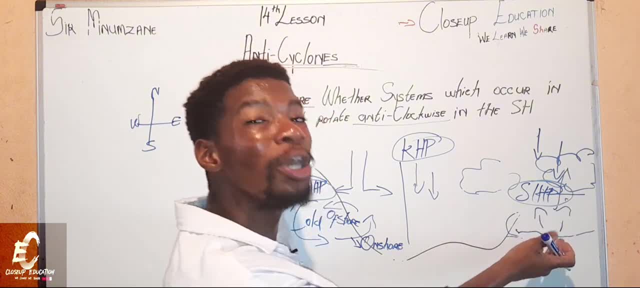 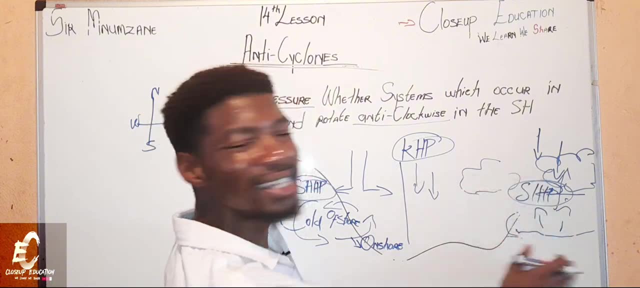 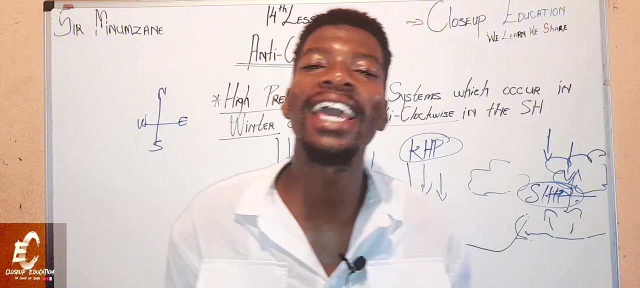 it prevents this smaller moisture air, which is already on our indian ocean, from trying to enter our land. right, it prevents it. it's called the blocking cell, all right, obviously, if this high pressure cells is given a name, definitely this one has to be given one. this one is called the. 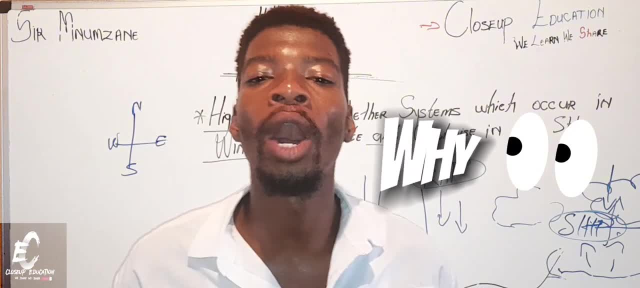 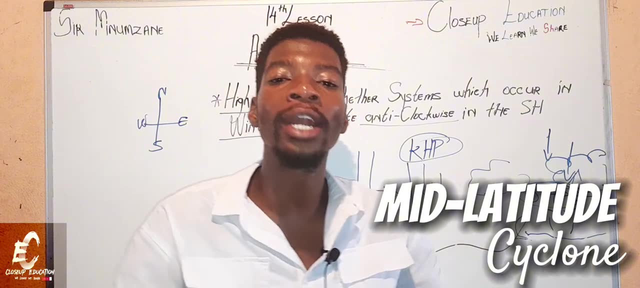 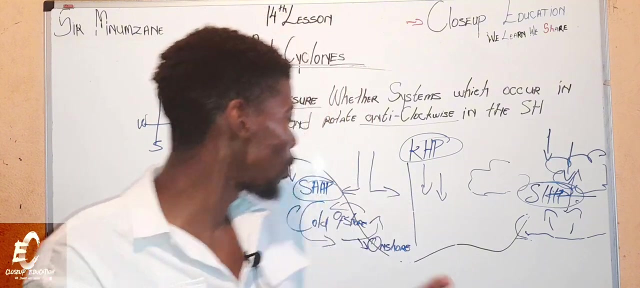 reaching cell. why is it the most important one? because of we know that mid-latitude cyclone, which i spoke about in the video before, this one also affects south africa in winter. right, it also affects south africa in winter. so when we have this south atlantic high pressure cells in the 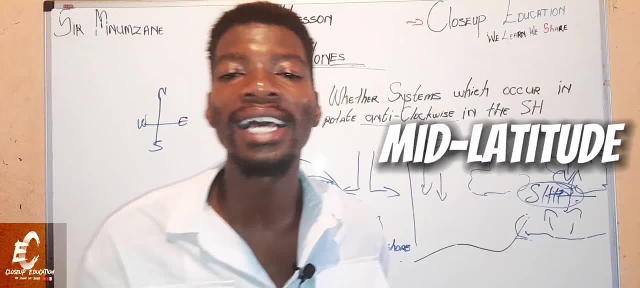 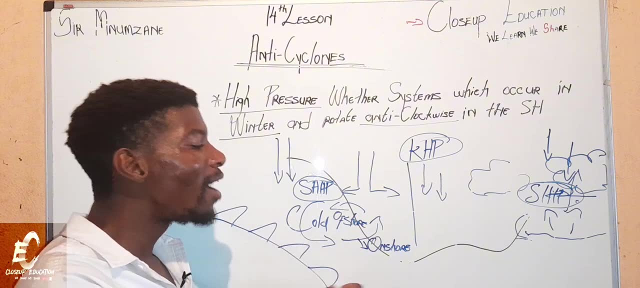 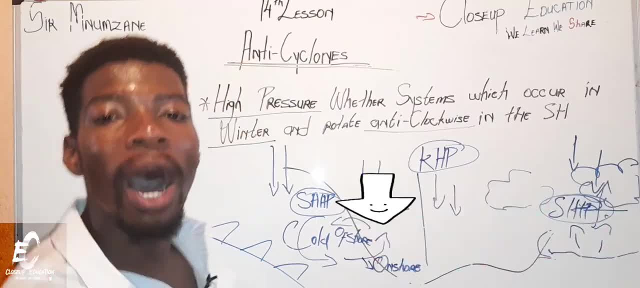 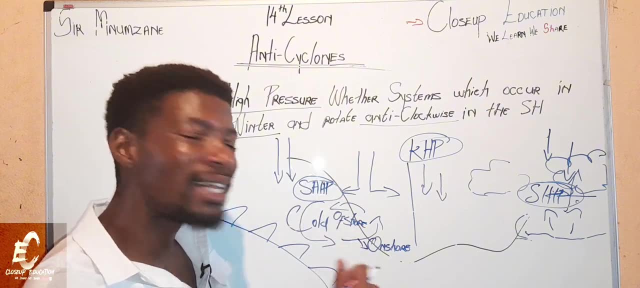 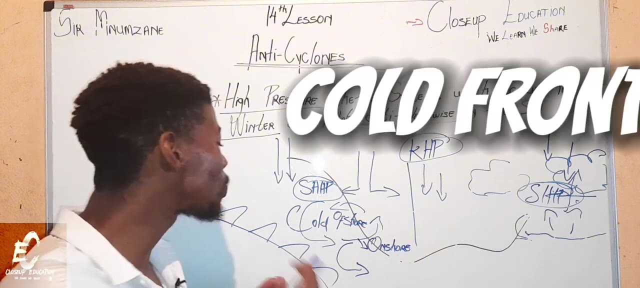 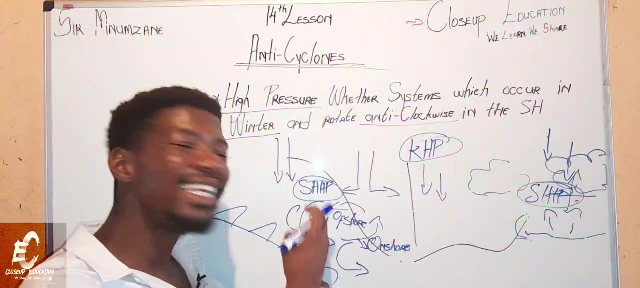 it will obviously be deflected further south. why will it be deflected further south? because of- remember- our south atlantic high pressure belt. it is a high pressure belt meaning it is rotating anti-clockwise. so when this cold front tries to approach our western cape, this south atlantic high pressure will reach or 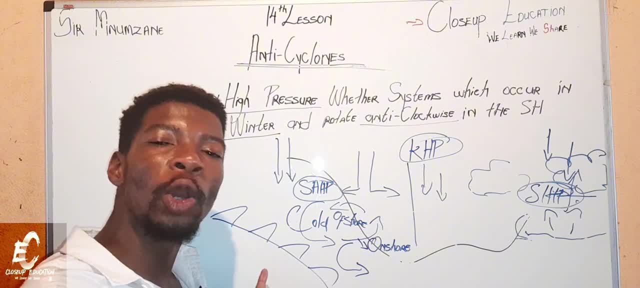 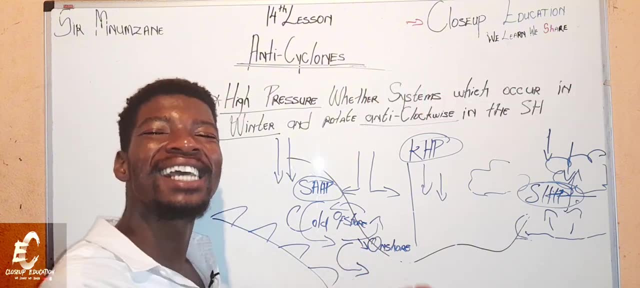 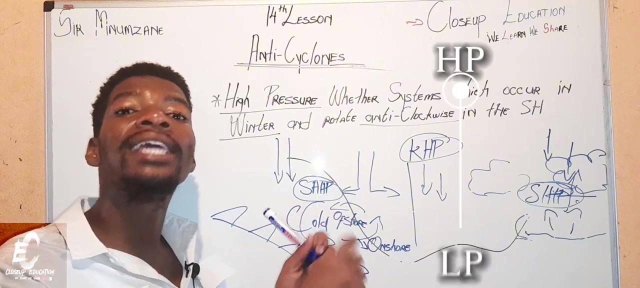 deflect the mid-latitude cyclone or the cold, cold, cold front from coming into western cape. so it will deflect it anti-clockwise because of we know that it is a high pressure and mid-latitude cyclone, it's a low pressure and we know that. 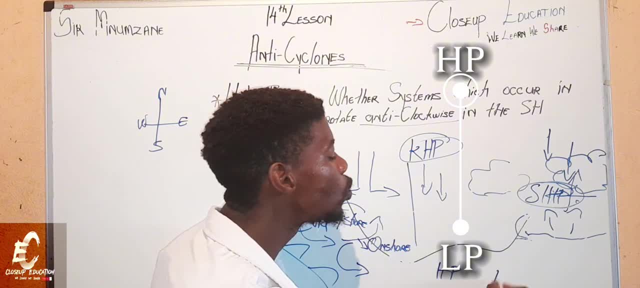 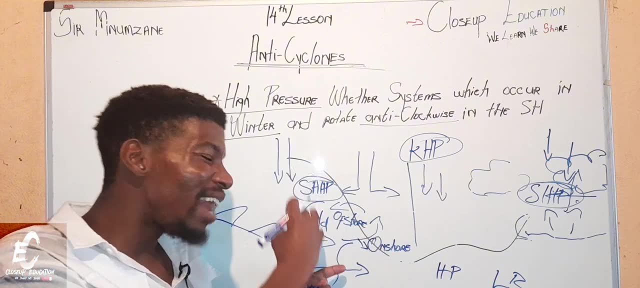 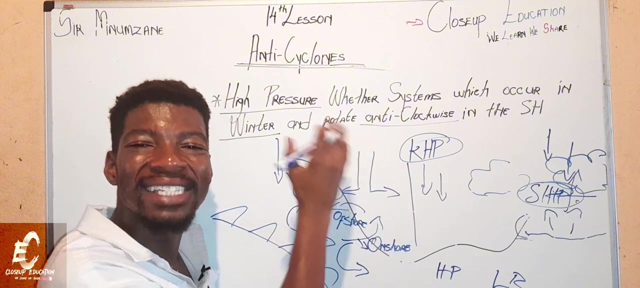 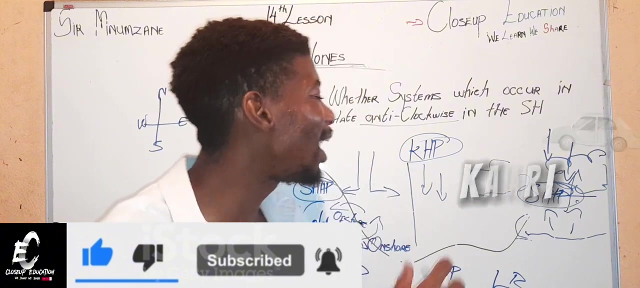 air moves from a high pressure area to a low pressure area. so when it tries to move to a high pressure area, it will be deflected to move to a low pressure area, not in an area where there is a high pressure. okay, before i could close this lesson, i obviously have to go to our kalahari. 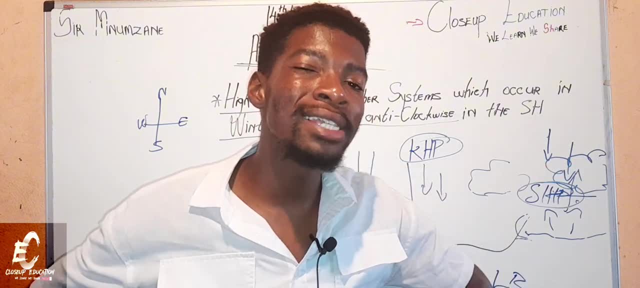 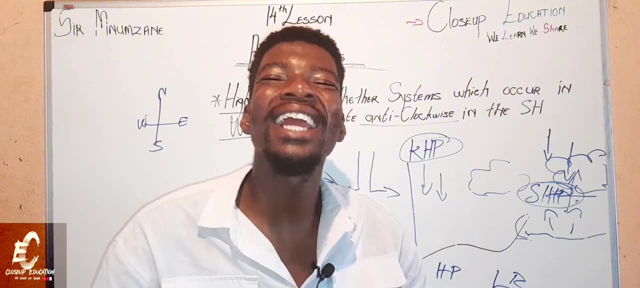 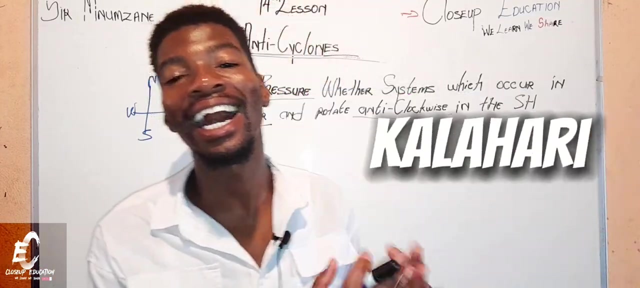 our kalahari. it is the most important one. i was thinking of skipping that one, but then i have to do it. okay, let me wipe this thing and try to explain kalahari at its best. four, four, okay, okay, in order for us to better understand kalahari, we obviously have to draw. 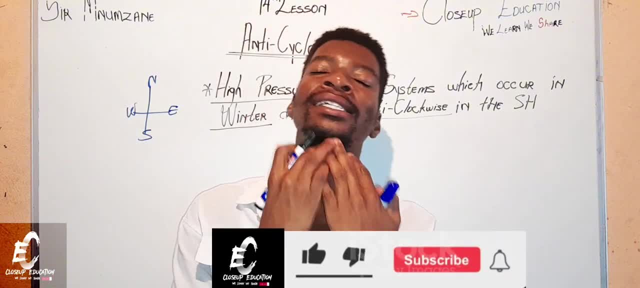 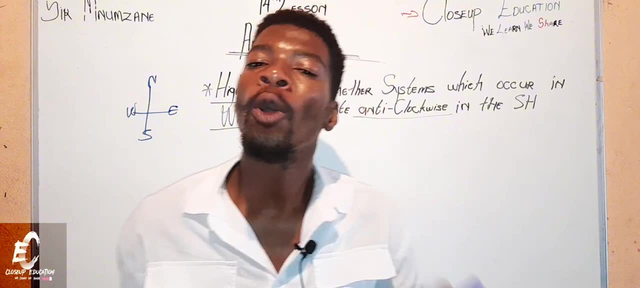 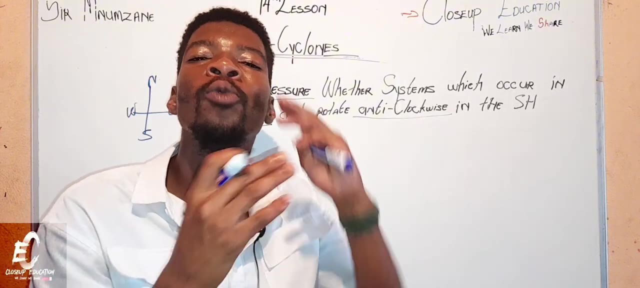 a piece in a sketch guys: geography. it is nice. you have to like this video. subscribe to my channel because of i'll be bringing you the joy of geography. once you know one thing, you will definitely know the next. all right, so this is winter. we'll obviously begin with the winter. 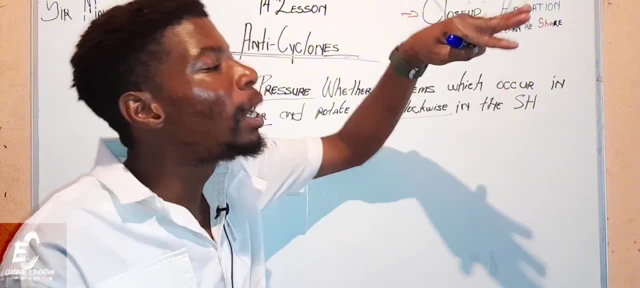 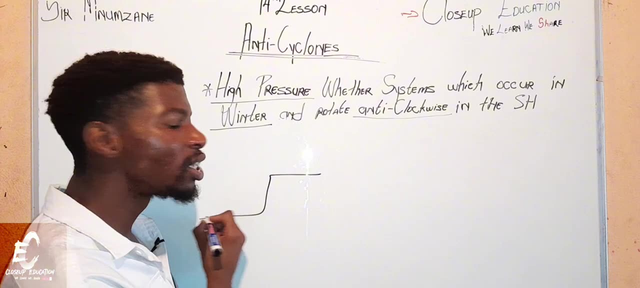 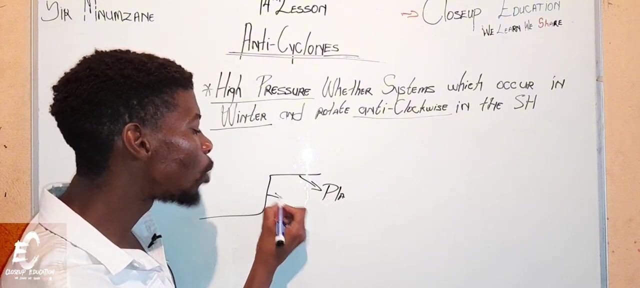 so in winter the kalahari high pressure will move further south. it will move towards our plateau. so our plateau, it is obviously what we call our land. so this is what we call our plateau, right, this is our land. and this is what we call our escarpment, right, this is our mountain escarpment, all right, and here we have what? 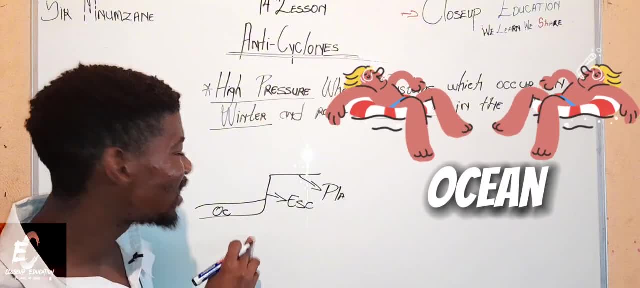 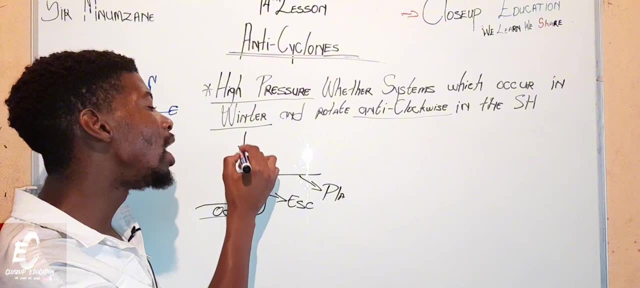 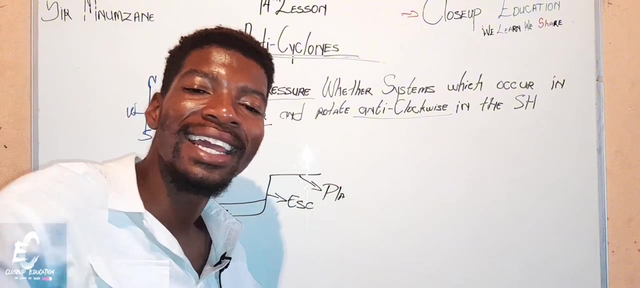 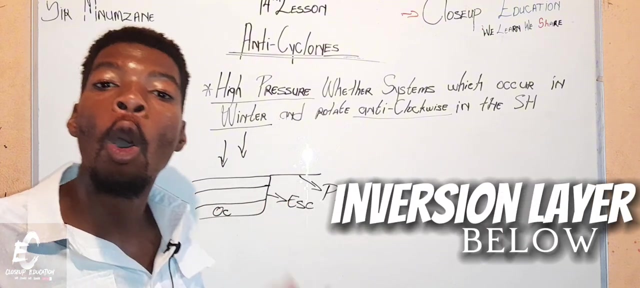 we call our very own ocean. right, this is our ocean. so we know one thing: that this it is winter. so in time there is what we call descending air. right, so the kalahari, it is obviously influencing the descending air. so, meaning the mountain, we will have the invasion layer below the escarpment. 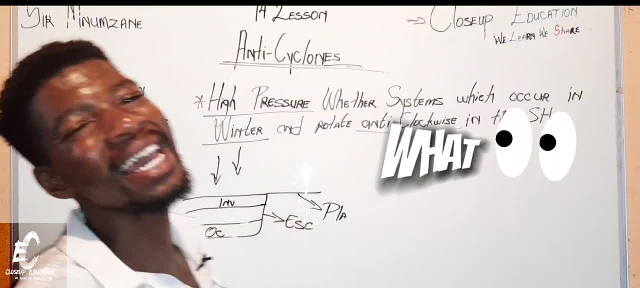 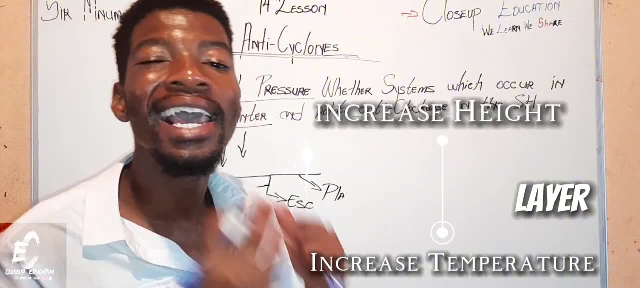 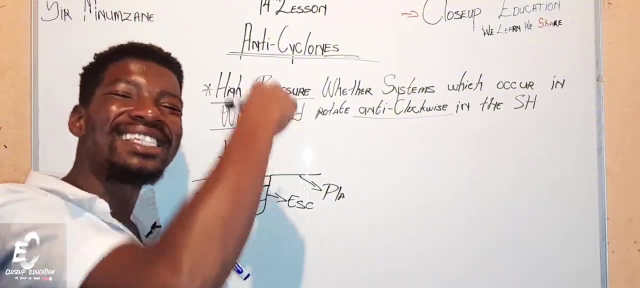 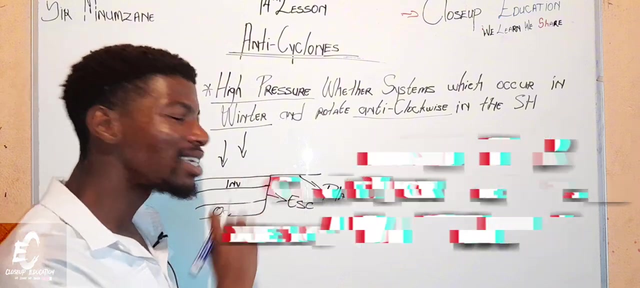 this is what we call the invasion layer. what is the invasion layer? the invasion layer? it is the layer which increases its temperature as it increases its height. so its temperature increases as it increases its height. so, because of there is descending air, this area will obviously be forced to not increase its height, so it will obviously be below the escarpment. so 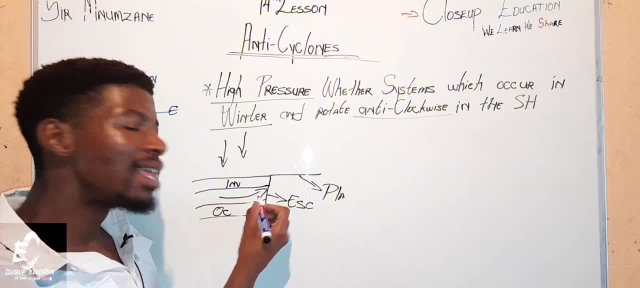 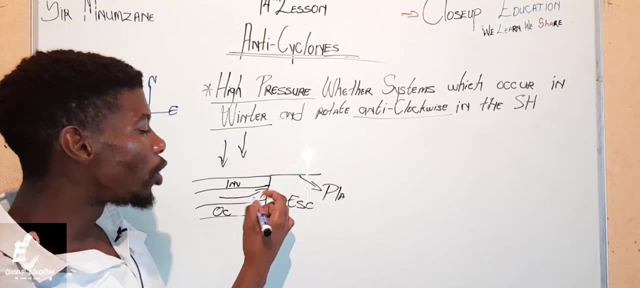 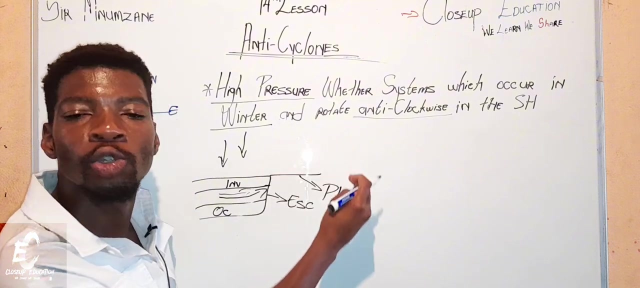 what will obviously happen to the air coming from the shores? it will obviously not be able to enter our land, so this area will not be having any air entering, or small air entering our plateau. this is winter, our kalahari. it is here. it forces the invasion layer to be. 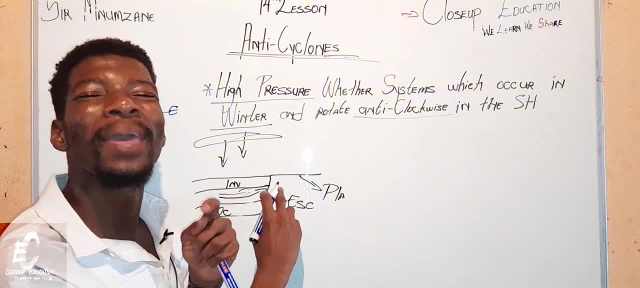 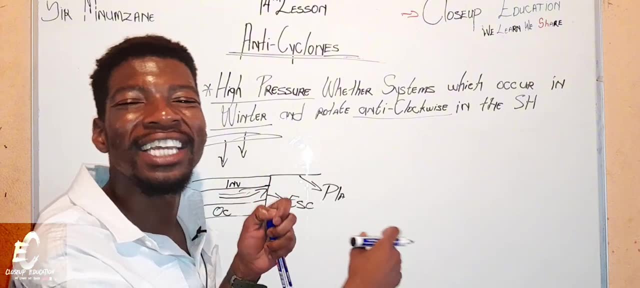 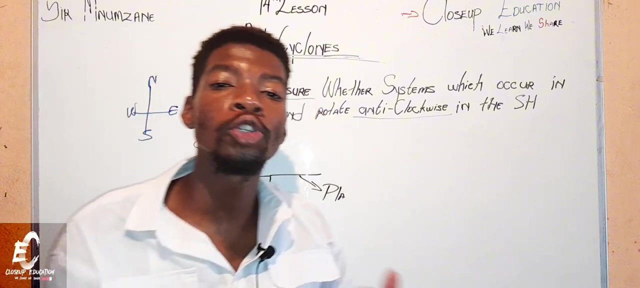 below the escarpment, so that there won't be some air coming from either the indian ocean or the atlantic ocean. so there could be some precipitation or community numbers, clouds. but then what happens? if we are not talking about winter? yes, if we are talking about some, our kalahari will obviously do. 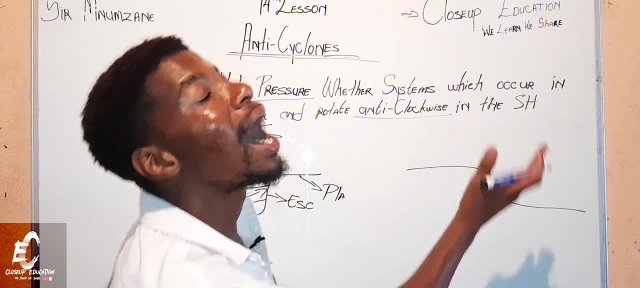 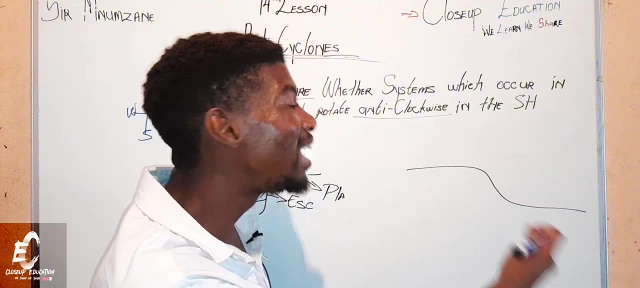 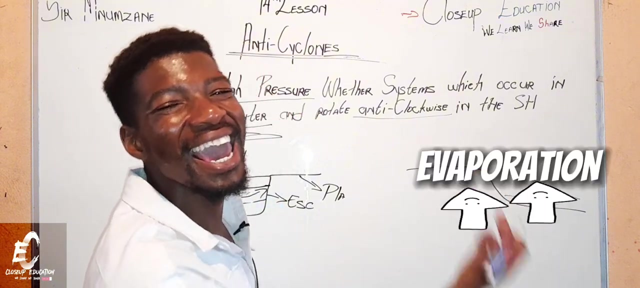 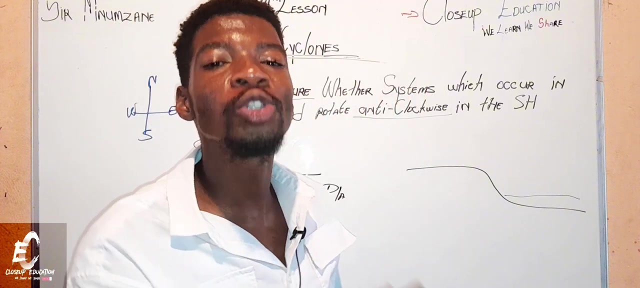 the opposite. it will obviously move further north. why further north? because of there has been direct insulation from the sun hitting either our plateau or our ocean, so there will be obviously what we call rising air. so the rising air will force the kalahari to move further north, right, 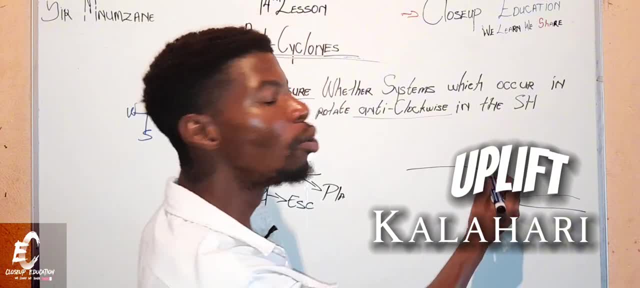 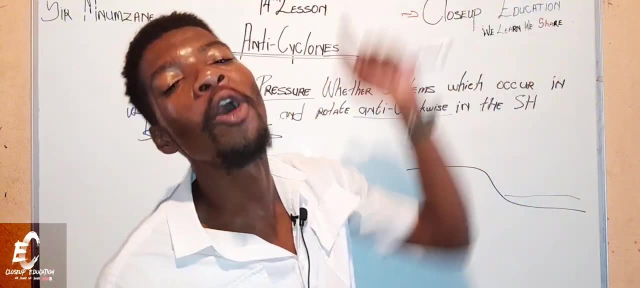 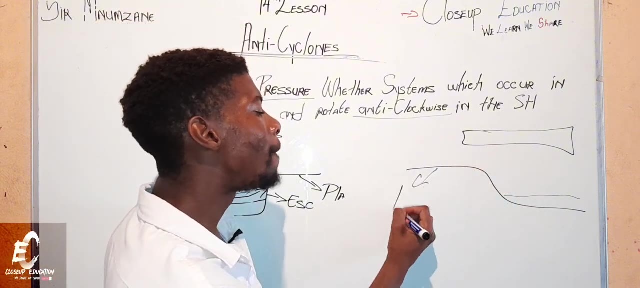 so the rising air will force the kalahari to move further north and obviously, if the kalahari is forced to move further north, even the invasion layer will be forced to move further north, so our invasion layer will be here. so this is our obvious what we call plateau, and this is